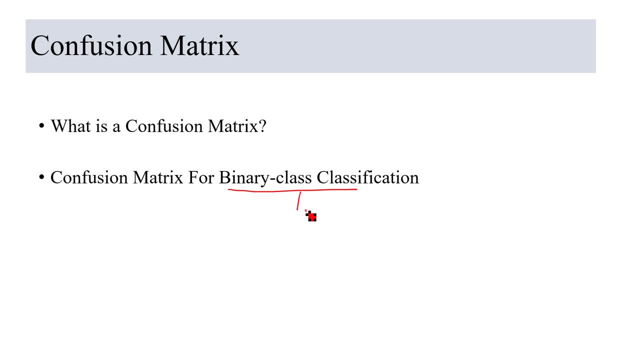 So if the target variable has the only two classes, that is, the zero or one, or positive, positive or negative, or male or female, yes or no, like this, only the target variable have the only two classes. two classes means either zero or one positive or negative, like that. 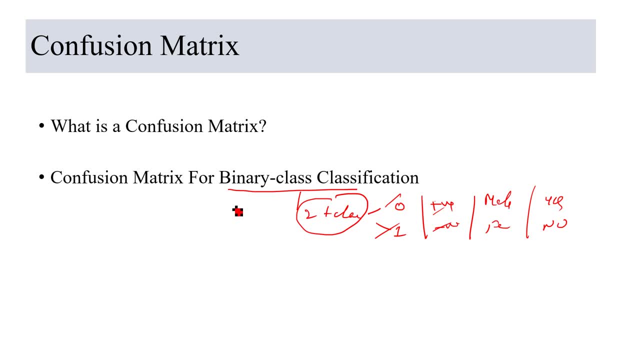 If it is more than two classes. that is the multi-class classification. So in this part one we are going to discuss about the only binary class. So in next lectures I have to discuss about the multi-class. So what is the confusion matrix? So confusion matrix is a. 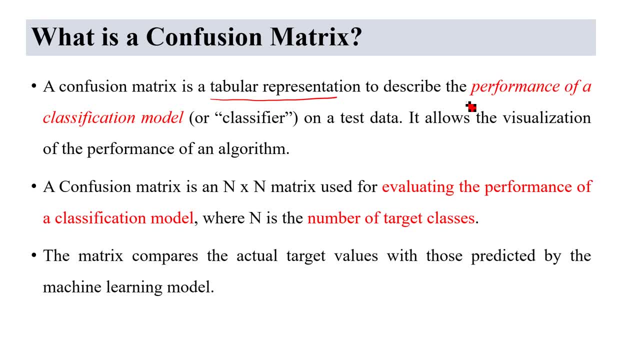 tabular representation to describe the performance of the classification model or the classifier on the test data set. So what is the test data set? So already in my previous lectures I already explained, I already described the test data set. even now I will also again. 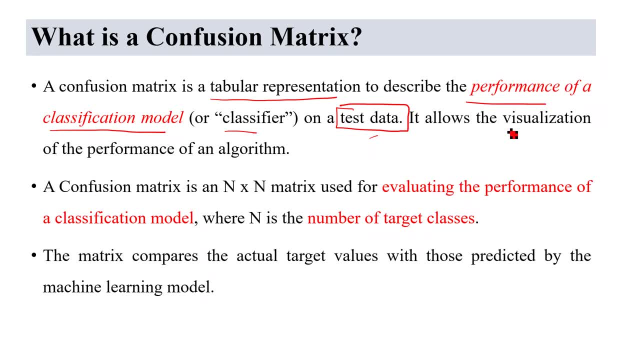 explain the test data set and it allows the visualization of the performance of the algorithm and the classification of the algorithm. We will get the final version of the, the information, when we will know the result of the classification process. So next one, it is the confusion matrix. the contribution matrix is the n by n matrix. 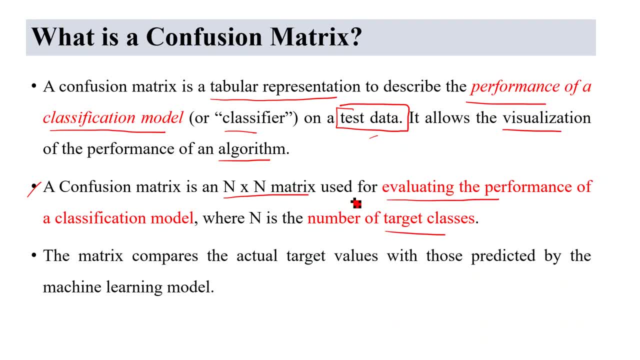 it is used for the evaluating the performance of the classification model. So what is the n? So n is nothing but the number of target classes. Suppose the binary classes, that is the 2 by 2 matrix. So n means there are the only two classes, that is, the either zero or one. If it is three by three matrix means 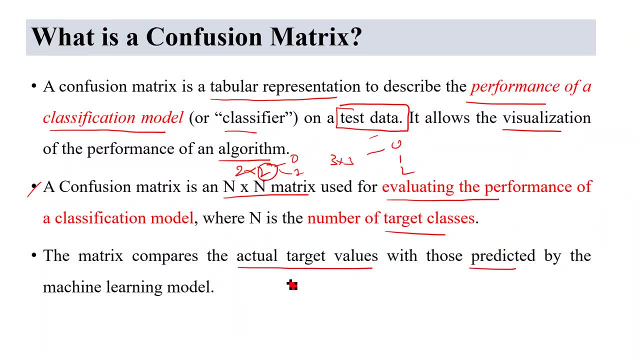 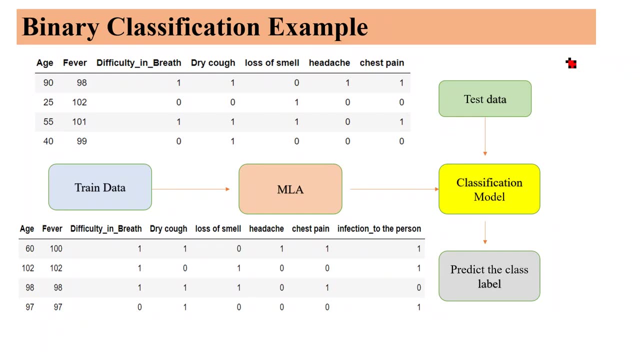 target values, with this predicted by the Michelin models. so means that we have to compare the actual target values with the predicted values by the model. so if you see this example, actually the data set shape is 1000 comma, 8 thousand rows and 8 columns, so the data set is divided. 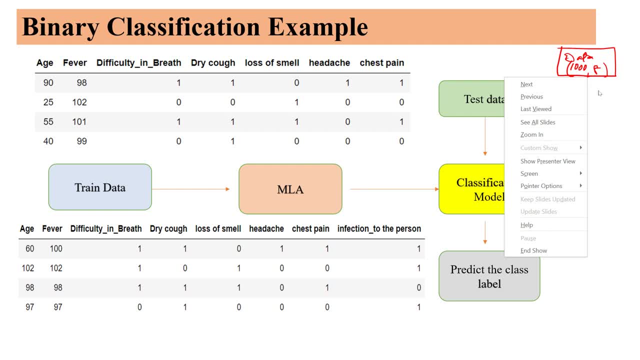 into two parts means like that: X and Y. so X and Y means so this is the input variables. why is the target variable? so here the entire data set of thousand rows of 8 columns. we are divided into training data and the test data, so suppose I'm considering eight, ninety. 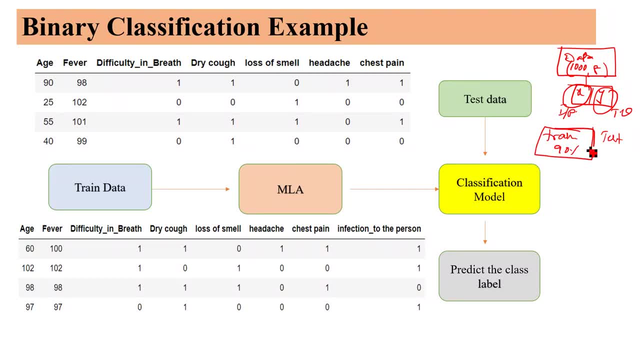 percentage of the different relation for that column. so for subject there is not zero. So it says I am a test computer. like in the test I will personally test up advanced what we have to use for the trainer model and just a 10 percentage of the data we have. 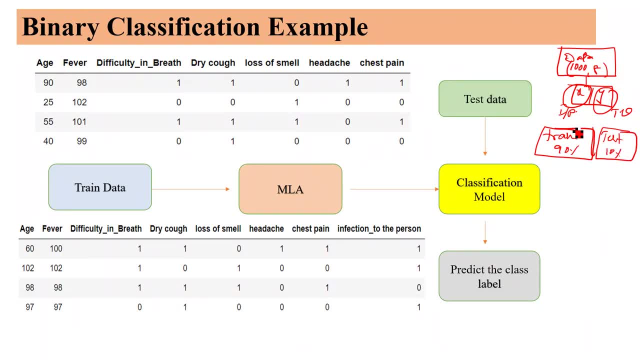 to use it as the model. so in the training data X and Y, both are existed. so in the test data also X and Y are existed, so in it. so here in this, 90 percentage of data means like that: this is the 90 percentage of the data, so here. 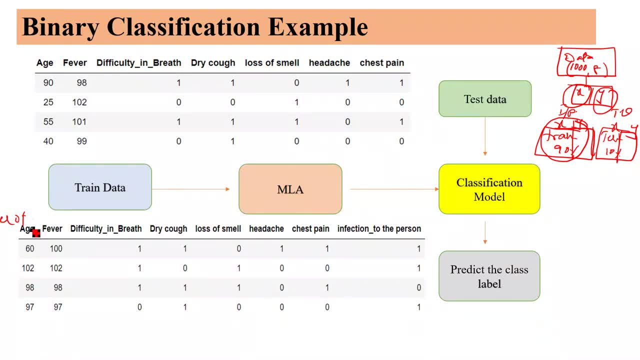 how many features are existed? the- this is the feature one- X, 1, X, 2, X, 3, X, 4, X, 5, X, 6 and X our. so they are the 7 input features. this is the target feature. so this target feature has the only two wellies, that is, ones, and zeros, only two. 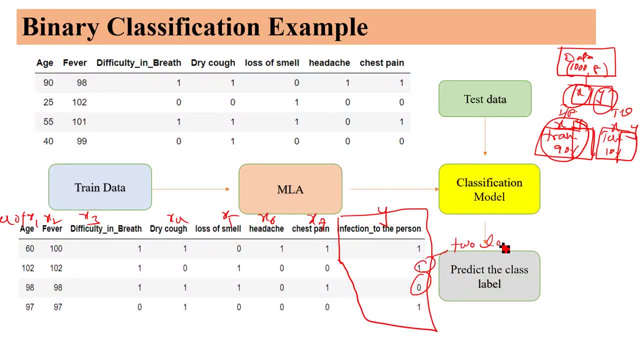 classes. so these are the basic class. this is the target features only two classes. that is the binary class. so what is this problem? so this is the data set about the whether the person is suffering from the disease, like nowadays, people are suffering from the corona. so how can you classify the? 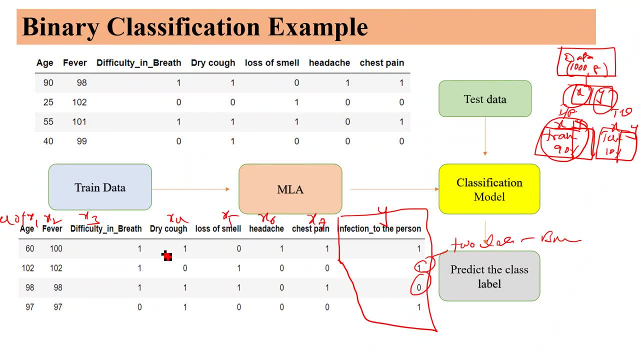 person is suffering from the corona or not. so based on this, some input features means based on some parameters. so suppose based on here there is seven parameters, x1 to x7. so based on age, fever, difficulty in breath and rake of loss of smell, headache, chest pain. so age means number. so this is the input data. 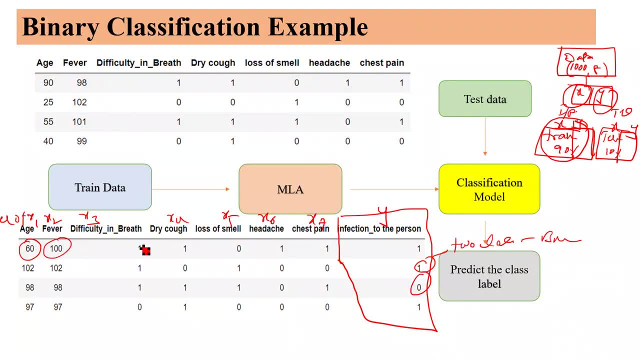 fever, so difficulty in breath. one or zero. so one means is suffering from the breathing, zero is not suffering like that. so this is the. this is the dummy data set, not the exact data set. so, for example, purpose, I am taking this data set. so, based on these seven features, 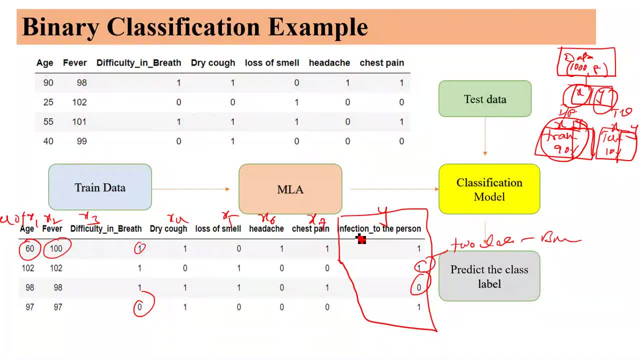 we have to classify the, whether the person is infection to the person, the corona, or not, yes or no. so this is the training data. so training data means this is the 90 percentage of data we have to use to the you can give to the machine learning algorithm. suppose I am taking the logistic regression, so 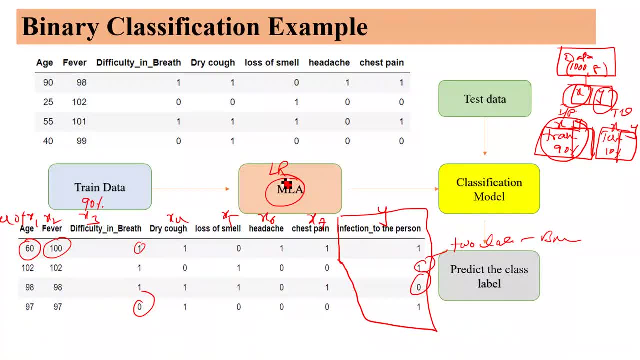 logistic regression algorithm are applied on the training data set. now we have to build the model, that is, the classification model. so next to what we have to do, we have to take the 10 percentage of the test data set. so in the 10 percentage there is only input features. see, if you see this is. 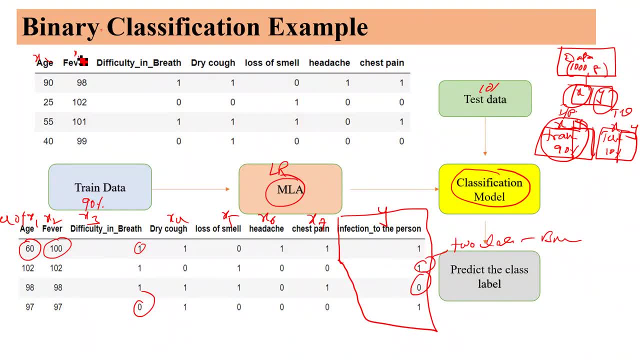 the X, 1, X, 2, X, 3, 4, 5, 6, 7, only input feature. there is no target variable, so only the test data set. we have to give this data to the model. the model will predict the labels means: predict the labels means this is the H bar labels. 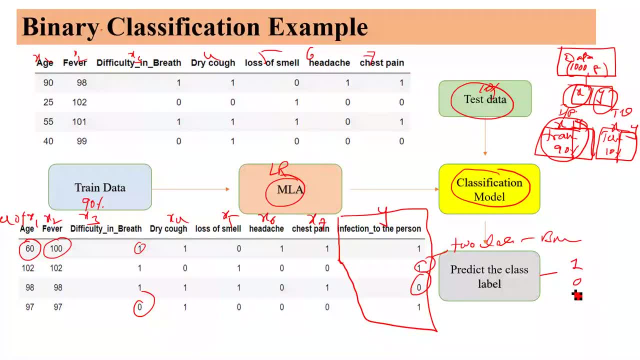 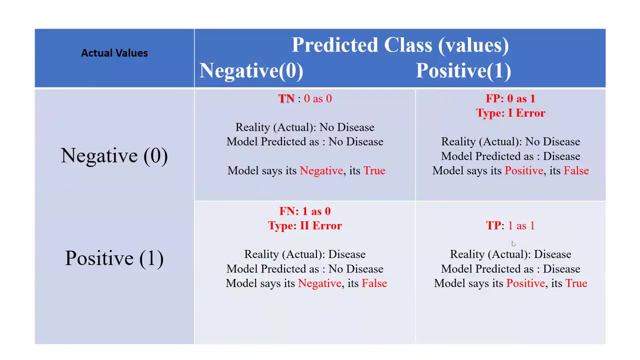 and model predicted the 1: 0 like that, based on the performance. you have the model. so, if you see, this is the confusion matrix. so in this confusion matrix, this is actually binary class. so binary class be divided into two by two rows, two columns, two rows, two columns, so on the 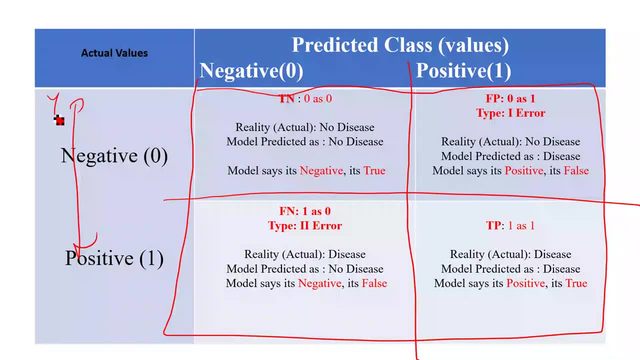 y-axis. this is y-axis. I am taking the actual values. on the X 6 I am taking the predicted values. so here negative means there is no disease. I'm cuz that I'm using like that. first two means is suffering from the disease. so actually means really the person has no disease. but here negative means the. 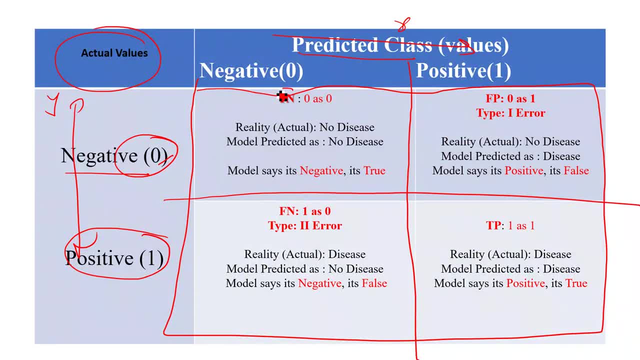 model practice negative. so TN means the true negative. so actually he is no disease model. also say that no disease, like that. so actually he is the no disease model, also predicted as no disease. so there is positive and there is no disease. so that is true means it means model says that 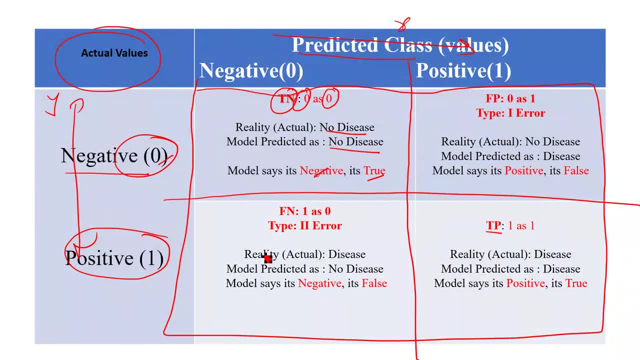 it is negative. true, so what is the TP? TP means true, positive. so H value has the positive, H value has the disease. so model also predicted as a disease means this is a true. is model predicted as a positive, is it true. so this is correct, correctly classified. this is also true, positive, true, negative, certainly. 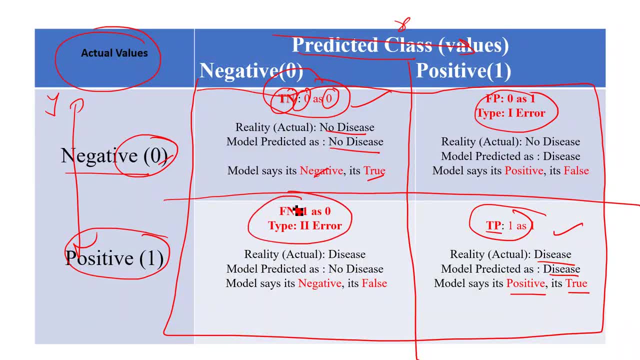 classified. but here FV and FN. these are falsely predicted means to TP. FV here if as negative, 0 as negative means that actually he is the negative, but protected as the one that is the type 1 error means he actually has no disease but model protected as a disease. that is the. 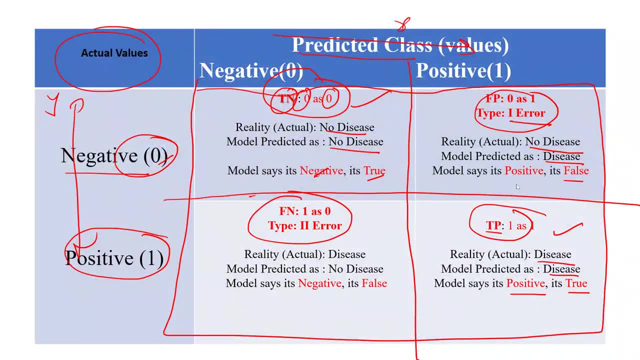 falsely protected. so this is also f2. fn is also type 2 error, which is falsely protected. really, he is suffering from the disease, but model predicted as no disease. so this is the error, means false negative is the type 2 error. false positive is the type 1 error. 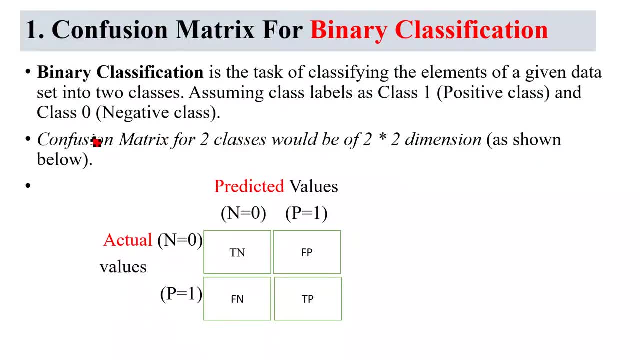 so confusion matrix for the binary classification. so binary classification is a task of classifying the elements in the given data set into two classes, two classes, zero or one. so among the two class labels plus one as a positive class and plus zero is a negative class. so i'm assuming like that. 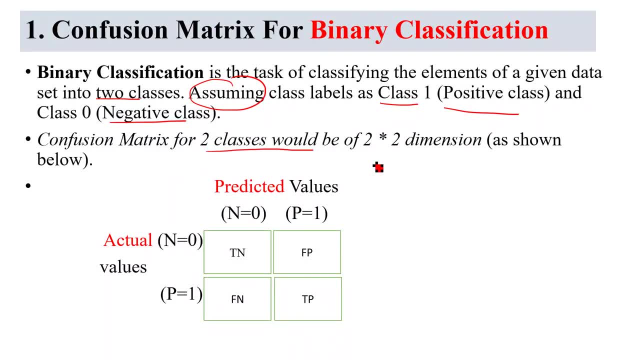 so confusion. matrix for the two class would be two by two matrix. so here, on the y-axis i'm taking the actual values, means n and means negative. so i'm considering negative is a zero, positive is equal to one. so on the y-axis and the x-axis i'm considering the um predicted values negative. 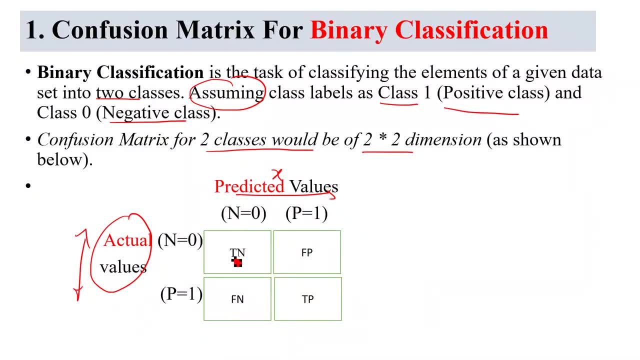 is equal to zero, predicted as one, so means the negative. negative means true, negative and negative. and positive is the true, false, positive and actually is the positive. and modipated as negative, that is the false negative, actually is the positive. and model also predicted as positive, that is the true positives. so the terminology is in the confusion: matrix, so that a target 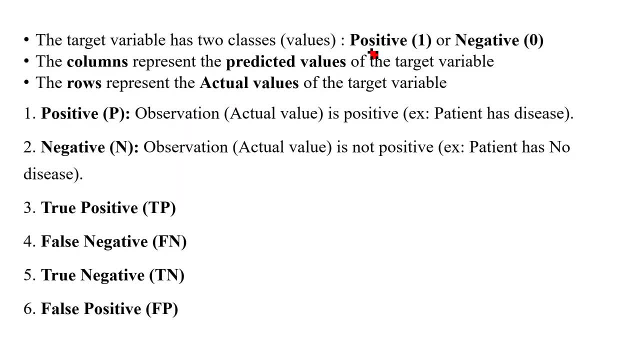 variable has the two classes. those are the positive. positive means one. negative is zero. i am assuming like that. so columns represent the predicted values of the target variable, rows represent the actual values of the target variable. so what is the positive here? so nowadays- this is the terminology is very famous- positive. positive means actually actual. 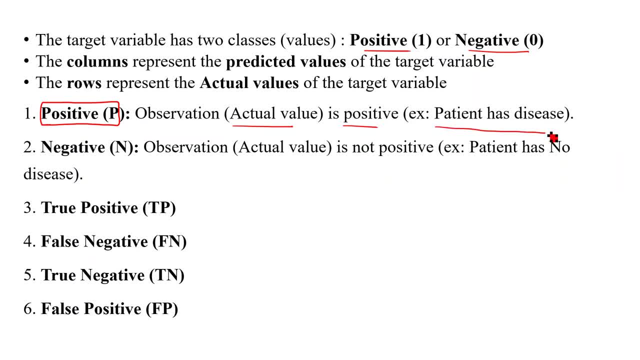 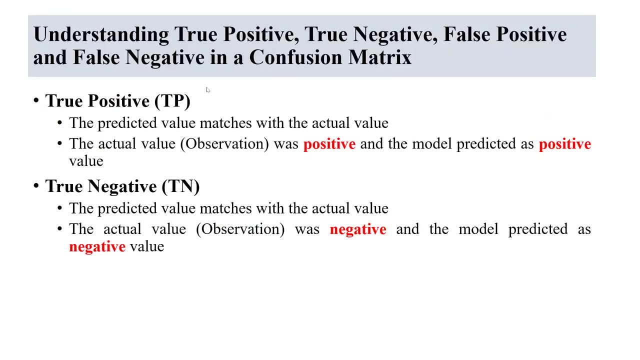 value is. positive means the patient has the disease. positive means person is having the disease. negative means no disease. and true positive, false negative. true negative, false positive. these are the terminals in the confusion matrix. so first we have to understand the true positive means. predicted values match the predicted values. 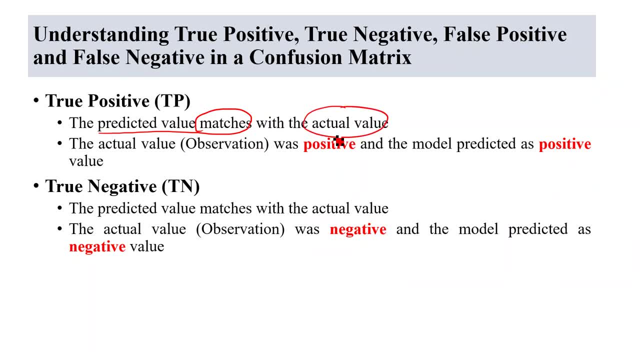 matches with the target values. so actual values means real values. so means the actual value means is positive. actually is the positive patient and model also predicted as the positive. that is nothing but the true positive. what is the true negative? this is also be matching with the actual values. so here actually person is negative and model predicted also be negative. 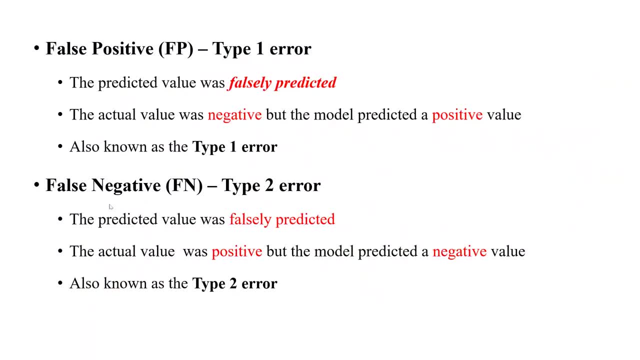 this is the true negative. false positive is the type 1 error. FV and FN means these are the falsely predicted by the modals means actually he is no disease. but model predicted as the disease means positive. that is the type 1 error. what is the type? 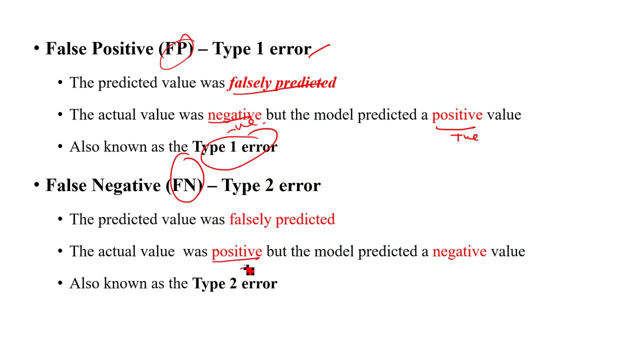 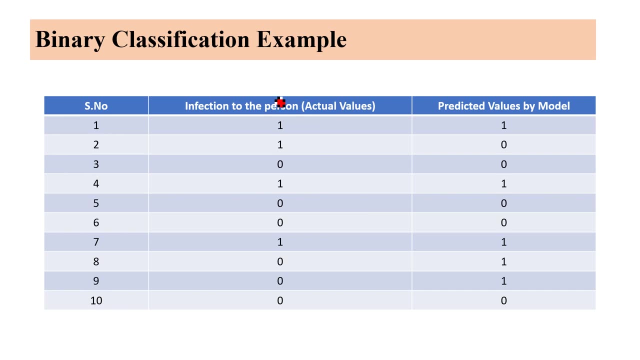 2. actually the person is positive, he is suffering from the disease and model predicted as the negative. that is, the negative means that is the type 2 error. so if you see the binary classification example, so here this is the our infection to the person. this is the actual. 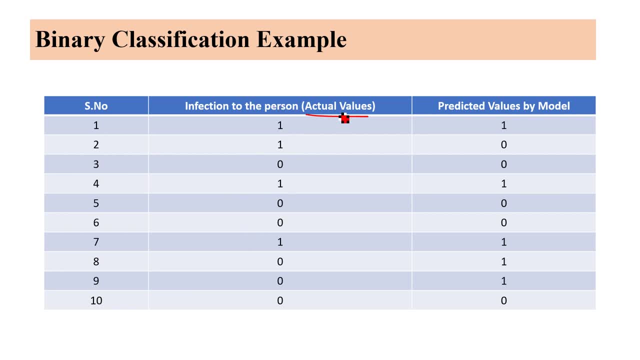 values, this is the our target values and this is the predicted values. suppose I am taking this example. so actually 1 is the 1 is the positive, 0 is the negative. so 1 is the positive and 0 is the negative. So actually he is positive patients, but model predicted also be 1, so it is correct here. 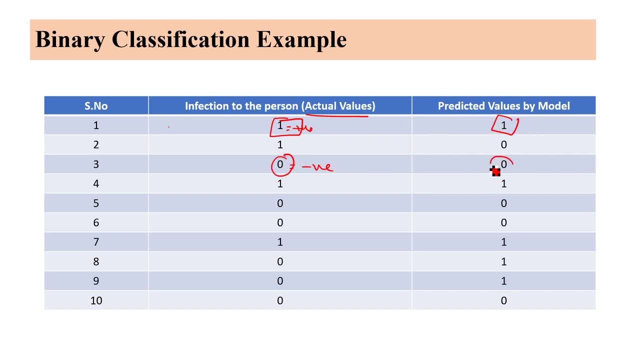 also negative model: predicted as negative. it is also correct. this is true, this is true positive and this is the true negative. but here, 1 and 0: 1 is 0 means actually he is the positive and predicted as the positive. 0. it is nothing but the 1 to 0. this is nothing but the false negative. so now we have to identify. 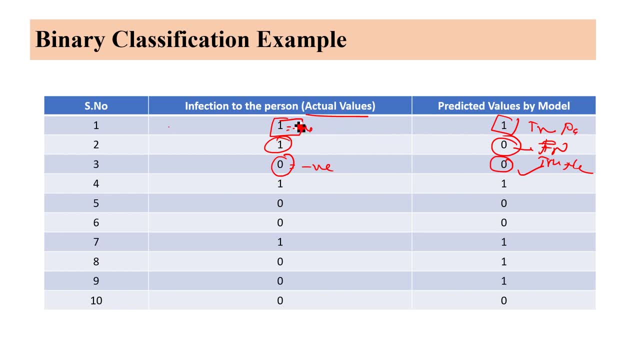 how many? 1. 1 to 1 means that. so here total number of rows means 10 rows, 10 rows. so how many? one to one, one to zero. zero to one, zero to zero. so here one to one means one one one, one, one one. so these are the one. two, one is three. so one, two, one three and zero one two. 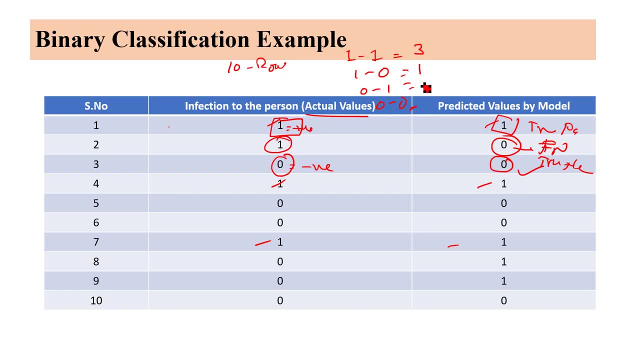 zero. one zero to one, two zero to zero, 4. if you submit 3 plus 1, 4, 4 plus 2, 6, 6 plus 4, 10, so these are the total 10 records 10 rows of the binary class, if you see after the 10. 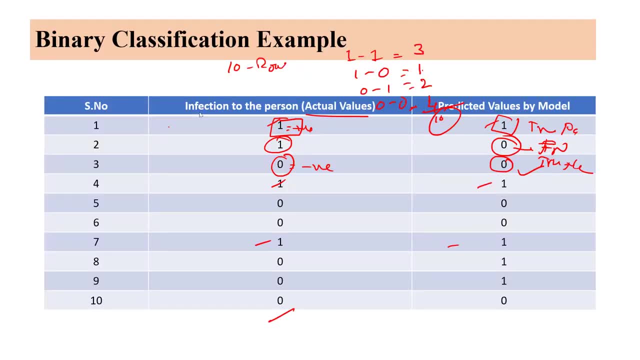 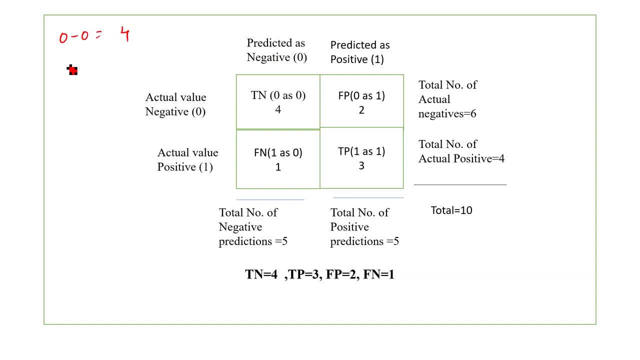 so in this example. so i'm considering 0 to 0, for 0 to 1 to 1 to 0, 1, 1, 2, 1 is now 1, 2, 0, 1. this is 1, 1, 2, 1 is 3, 3. so means here I'm assume that in: 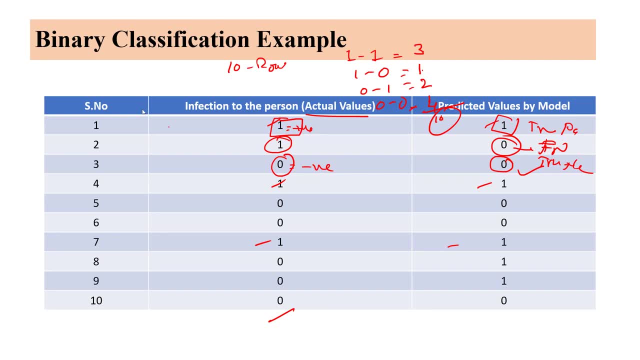 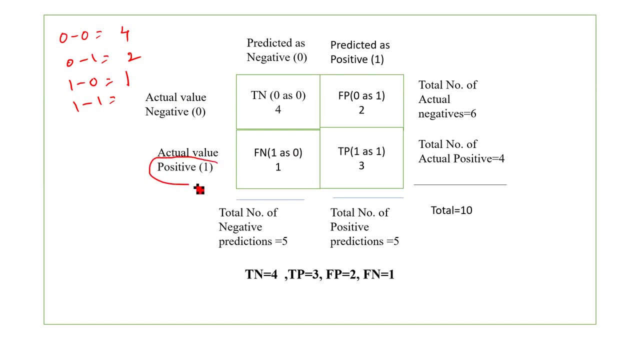 this example: 1 is positive, one is positive, so means 1 is positive and 0 is negative. this is my actual negatives and this is my actual positive. but here model predicted the negative, zero model predicted the one. so means how many zero zero, here zero and this zero matches how many zeros are zeros and zero. 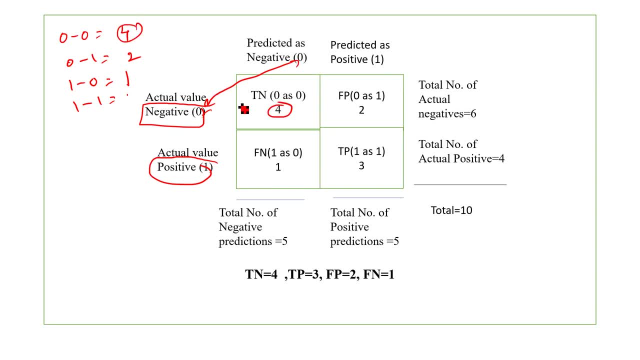 four. so this is the four. how many zeros to one? zeros to one. two: this is the two. how many ones? and zero. so actually is the one and model predicted: zero. that is the one and one and one that is the three. that's the true first. so i am assumed like that. so means out of the 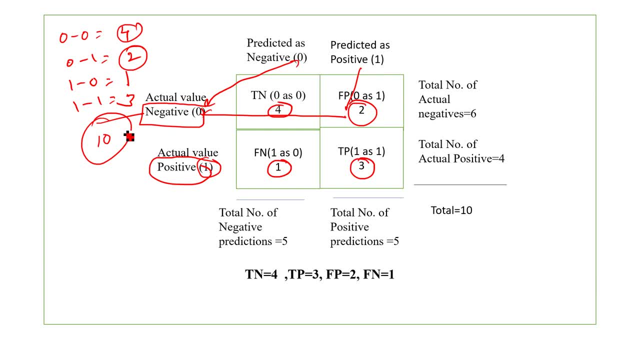 10 patients. how many negative patients? how many has the healthy person means negative, means he is, the healthy person means so total: six people are there after first 10. six people are negatives and out of 10, six are the negative. four are the positive patients among the four. 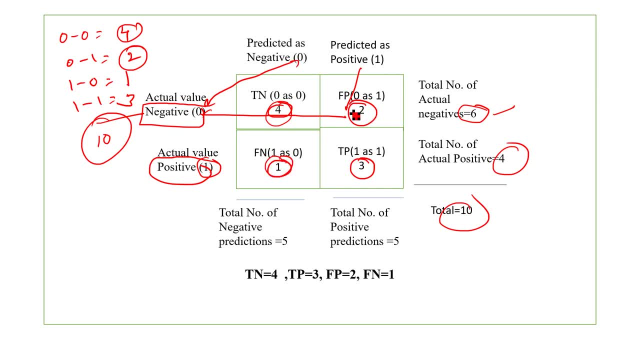 only one person is wrongly predicted and out of six, two persons are the wrongly predictors means for a correctly predicted. so that is nothing but the. so true negative false true p and true positive is three, fp is two and fn is equal to one. so what is the accuracy out of all classes? 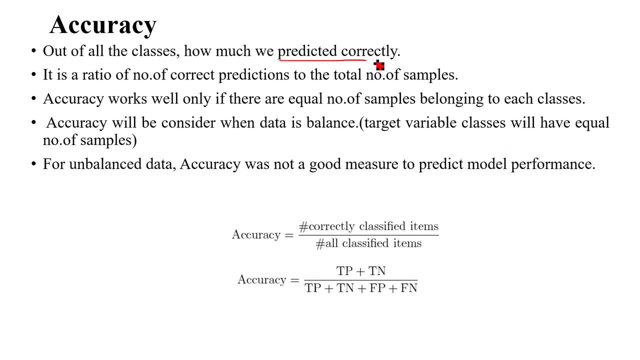 how much predicted correctly. how much predicted correctly means it is the ratio of the correct predictions to the total number of samples. means accuracy works well only if there are equal number of samples belongs to the each class. means that so thousand rows total thousand rows of the data set. 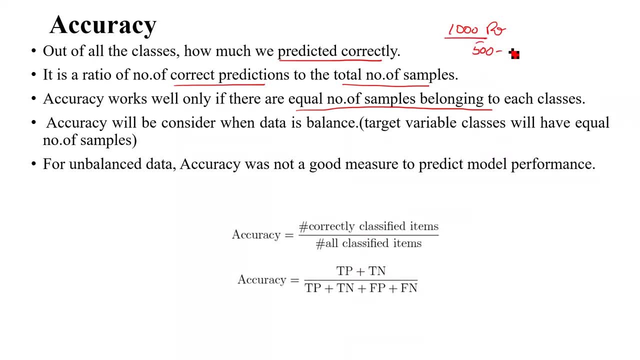 among the thousand rows, 500 rows are the positive, 500 rows are the negative- means equal number of the classes, one that is nothing but the same classes. at the time, only accuracy works well. if accuracy will be considered when the data is balanced, that is balanced: nothing but the. 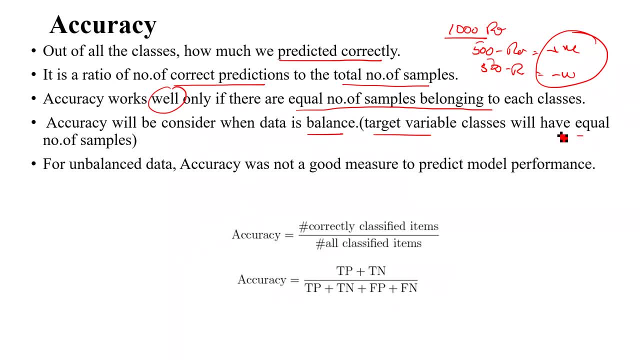 target variable classes will have the equal number of samples. equal number of samples means 500 positive and 500 negative, like that. so about to 50 to 50. percentage are the same sample. all are 40 to 60, like that. so in the two classes, one class is about 50 to 50 and 40 to 60 like that. this is the 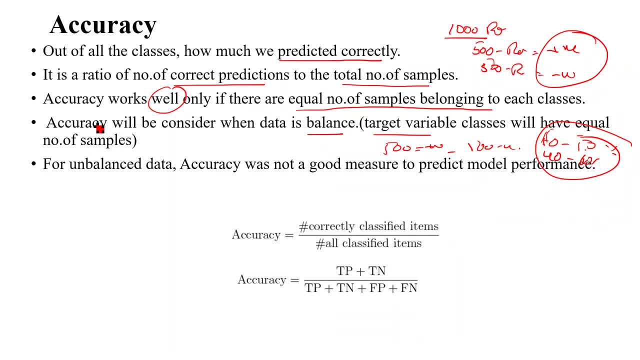 balanced data set for unbalanced data. so unbalanced data means suppose number of zeros is 900, number of ones is 100 means this is the unbalanced. so at that moment accuracy was not good measure. to predict the model performance, so to measure the model performance, so accuracy. 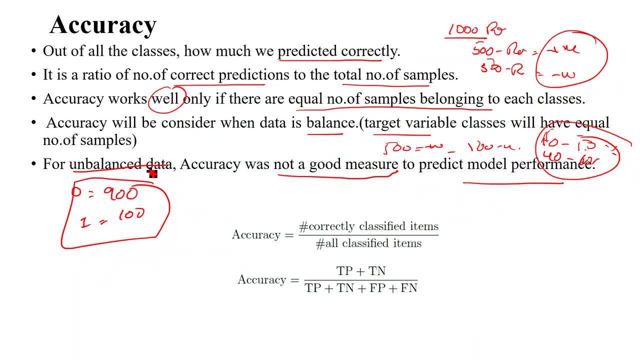 accuracy is make a key role. so if it is balanced data- 50, 50, 60, 40 percentage, like that, that is, we have to consider the accuracy if it is 0 to 1 or 90 and 90 percentage and 10 percentage kind of the 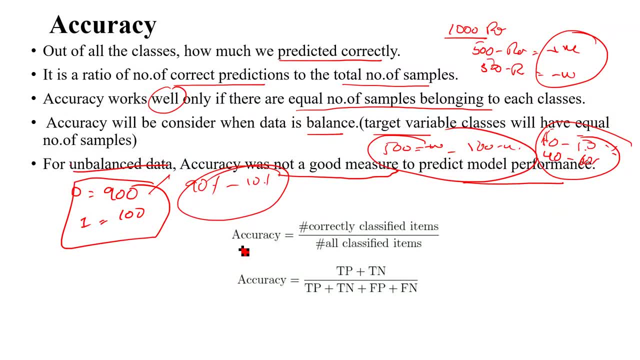 classes. we have to consider the unbalanced data set. so this is the formula. what is the formula? correctly classified items by the all classes items. so correctly classified items means true positives and true negatives are the correctly classified items by the all classifications. all means. so in this confusion matrix, this is the true negative, this is the true positive, this. 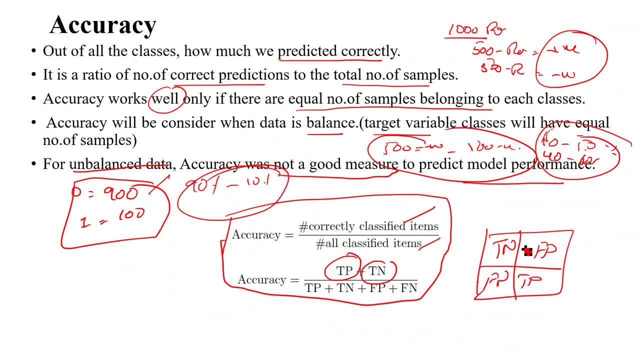 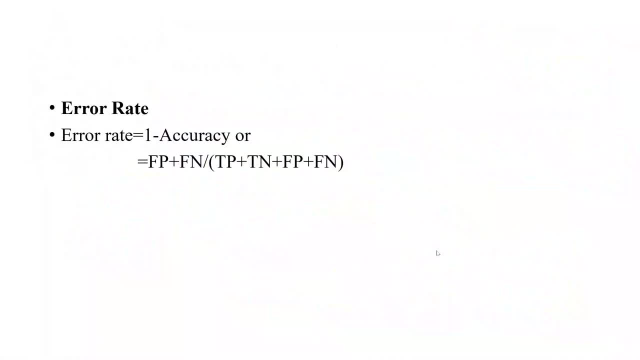 is the false positive and this is the false negative. so accuracy means tp plus tn by all items like that. so what is the error rate? so error rate is nothing but the 1 minus. accuracy like that means you can also write like that: incorrect predictions: fn plus fp by total. 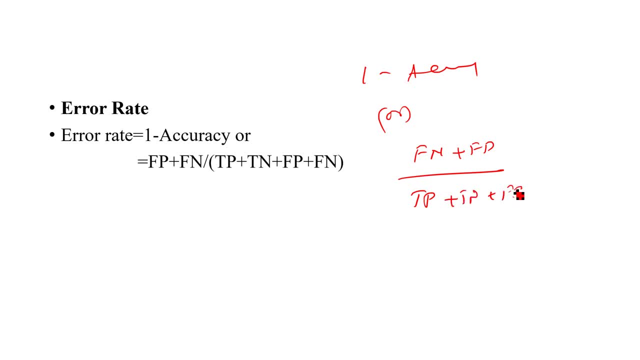 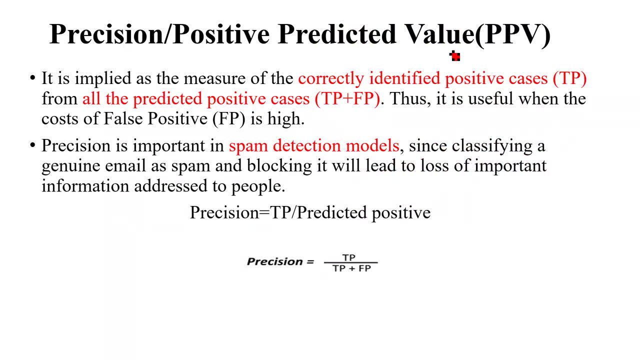 items: tp, tn, fp, fn, like that. so what is the precision? precision is another name- is the positive predictive value. ppb means that. so in this, this is the confusion matrix. so in this confusion matrix, if you write correction is a particular value, pp and pp it is the random phrases of an item. so these are the values of the particular points of the. 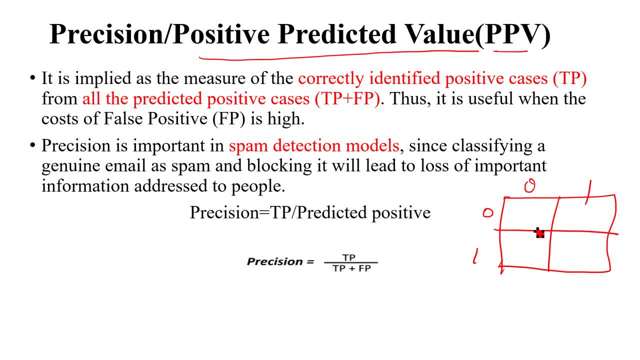 pp and pp. so the common phrases of the particular values, of the particular values here, is that, therefore, is 0, 1, 0, 1. so this is the true negative, this is the true positive. this is the false positive. this is a false negative, so means that it is implied as the measure the correctly identify the positive. 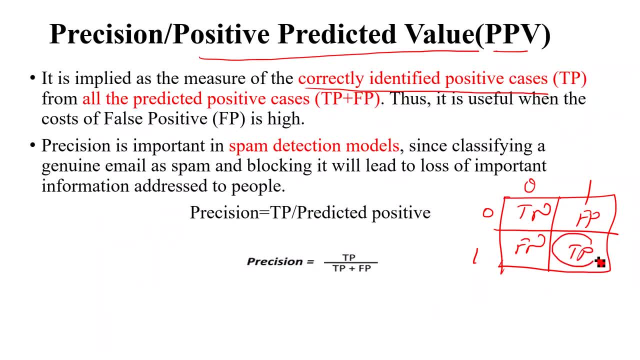 cases correctly identify the positive cases from the all predicted positive cases. all predicted positive cases means this is the predicted values and this is the actual values. so in this predicted values. so this part means tp plus fp is nothing but the predicted positive classes. predicted positive classes means tp plus fp. out of tp plus fp, how much we correctly identify means. 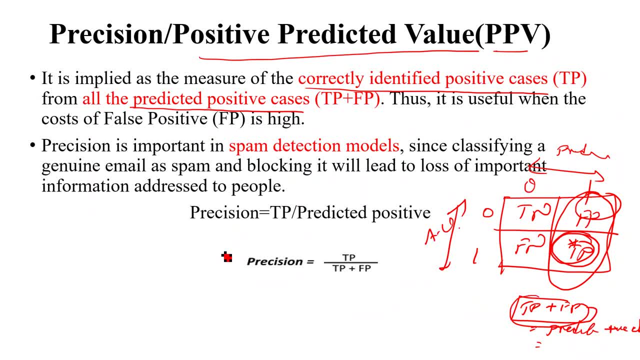 much. you correctly identified nothing but the tp. so that is the formula of the precision. precision means tp, this tp by tp plus fp. tp plus fp means this is the part indicating the predicted positive cases by the model. so precision is important. so in spam detection models, for example, we have to 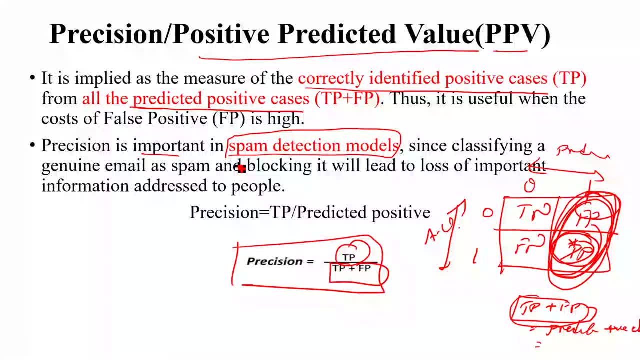 consider the: the given mail is spam mail or not spam mail. this is the scenario. so in this case we have to consider the precision. why? because by classifying the genuine email, so that is, the genuine email can be considered as the spam, and blocking it will be lead to the loss of some. 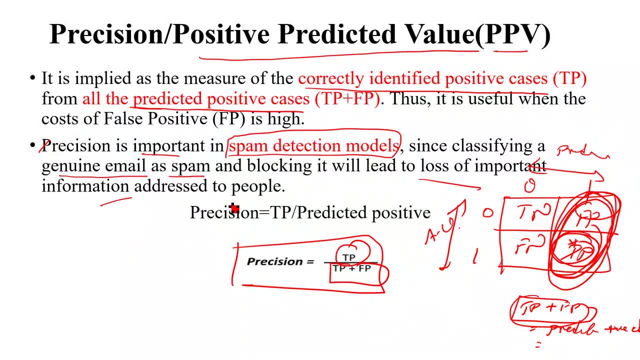 important information addressed to the people means that, uh, actually, this is the genuine mail. actually, this is the genuine mail, but it is also be predicted at the spam mail. so at that moment of time, people used to rather some important information. so this kind of examples, we have to consider the precision which is also 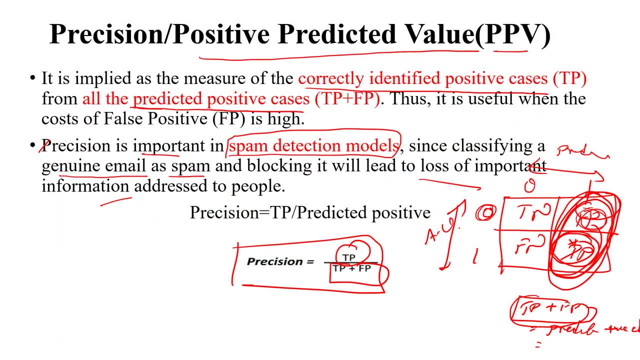 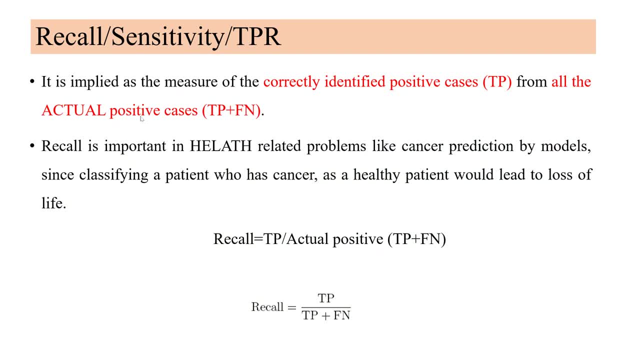 known as the positive predictive value. next, recall. what is the recall, which is also named the sensitivity, also known as tpr? tpr is nothing but the true positive rate, true positive rate. so it is implied that to measure the correctly identified, the positive cases means, in this confusion matrix: 0: 1. 0. 1. true negative. true negative. true positive. 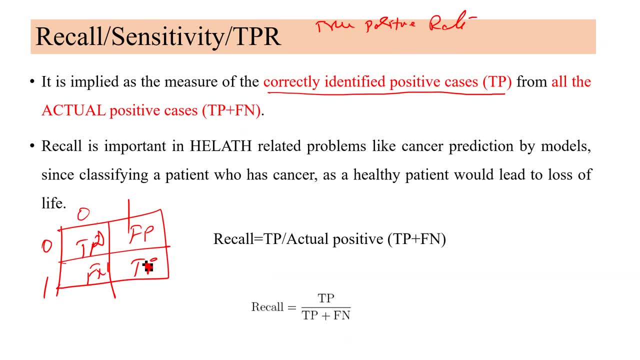 false positive. false negative so means that correctly identified positive cases. so this is the correctly identified positive cases from the all actual classes, all actual positive classes here. this is the actual negative, this is the actual positive. so actual all positive means this is the part that is nothing but the tp plus fn. 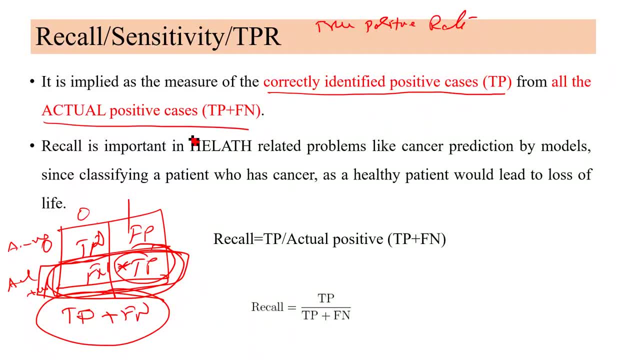 so that is the notation. so out of all actual positive cases, out of all. as to actual positive cases means tp plus fn. from this how model is correctly identified as positive cases. nothing but the tp means in recall is very important in health care kind of problems. health care means, suppose, cancer prediction, liver disease prediction. 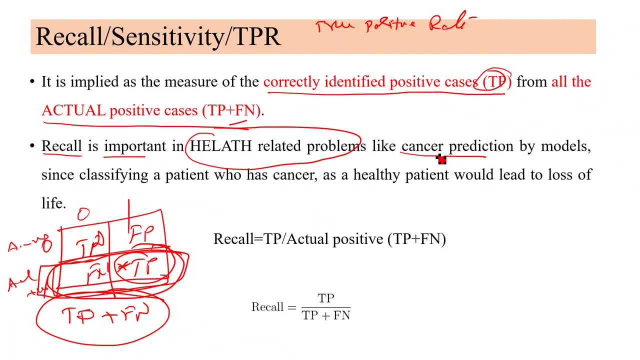 kind of problems at that moment of time we have to consider. recall is very important. for example, if you see, if you see in this case this is actually, he is the negative, nature is the positive and this is the negative. actually, this is the false negative. so in this case, really is suffering from the disease, but 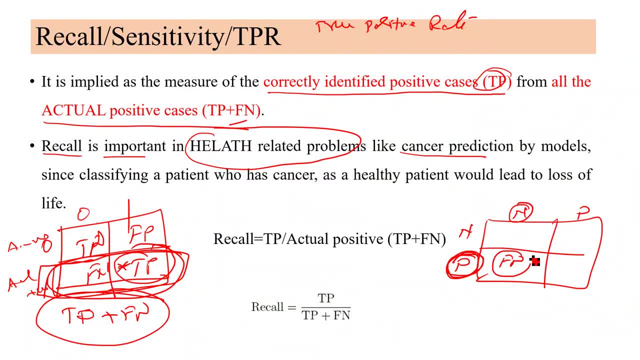 model says that you don't have disease. so that is nothing but the false negative. actually has the disease really suffering from the disease, but model predicts the negative, so means in this case, people lost the some life. so that is the nothing but the false recall, which is also known as the. 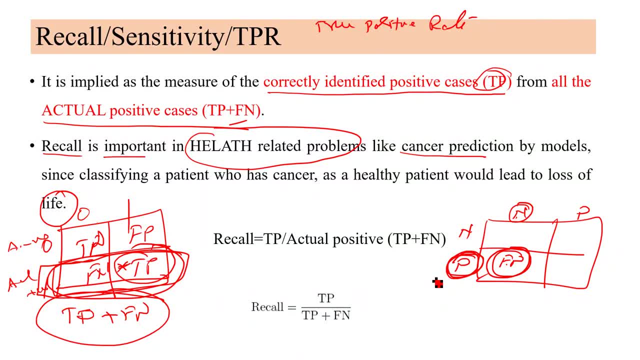 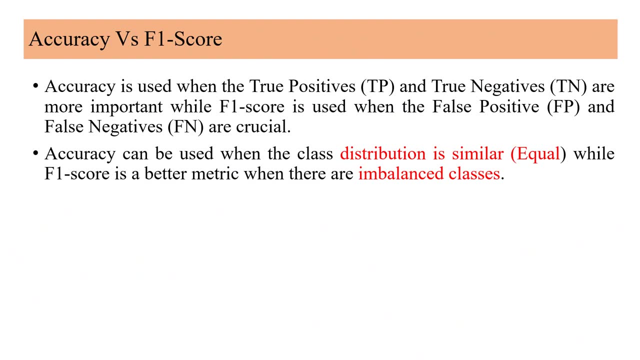 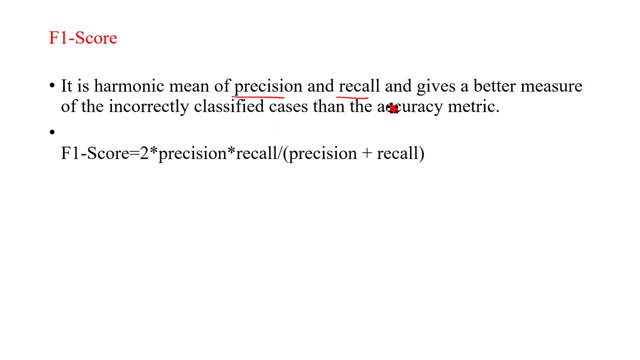 true positive rate, also sensitivity. so means that in health care kind of problem statements, recall is very, very important. so what is the accuracy and f1 score? so? so f1 score is the harmonic mean of the precision and recall and gives the better measure of the incorrectly classified cases than the accuracy matrix means. f1 score is nothing but the. 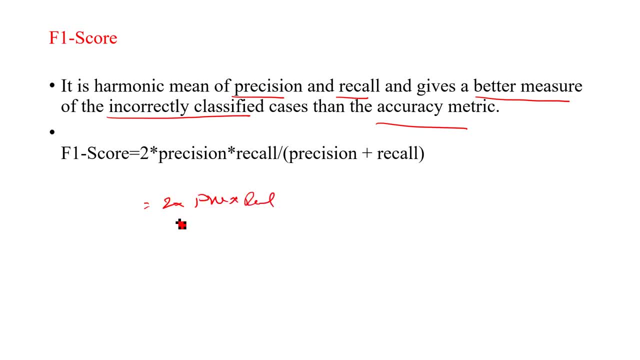 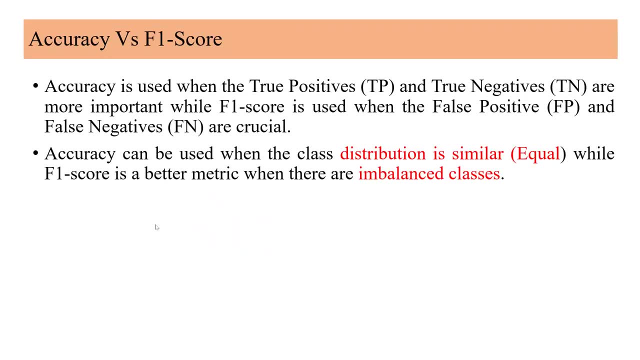 two into precision, into recall, by precision plus recall. so this is the formula of this f1 score. if you see, accuracy is used when the true positives and true negatives are the more important, while f1 score is also be used when the false positives and false negatives are the crucial. 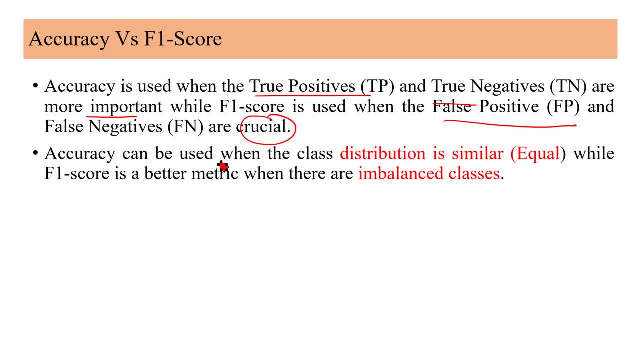 means accuracy can be used when the class is class distribution is similar. means equal number of classes. means this is the balanced data set. so balanced data set accuracy measure we have to consider. for imbalance data set, the f1 score will be considered. so this is the very 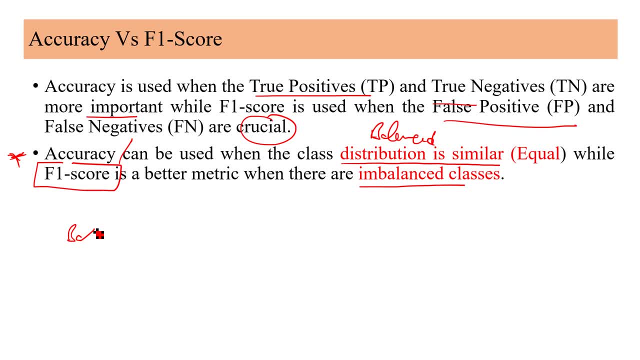 important point. so, based on, based on balanced data, based on the sub balance, based on the target variable, in the target variable, how many classes? so in target variables, suppose in direct, suppose 0 or 1, there are only two classes and zeros are 900 and one number of ones is 100. so 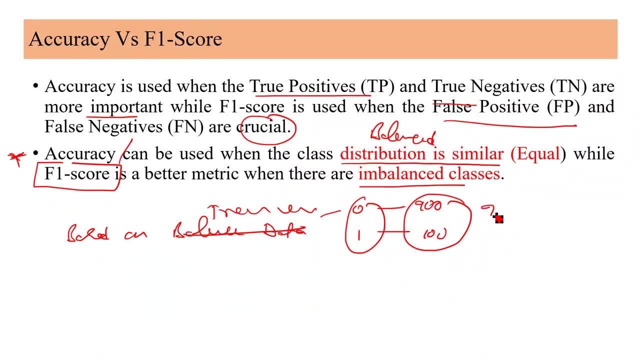 this is the imbalance in the imbalance, this is the imbalance data set. at that moment we have to consider the f1 score, suppose in binary class. so 600 are the positive means 0 and 400 are negative means 1.. so at that moment, this is the. 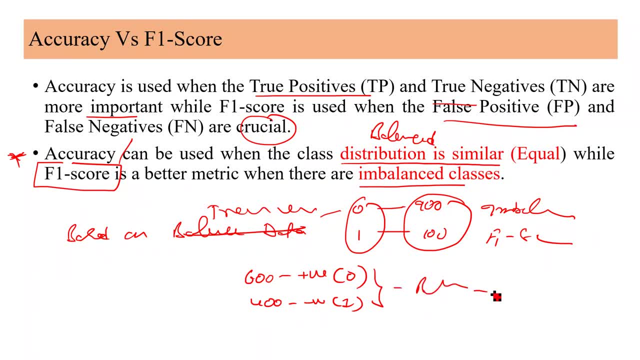 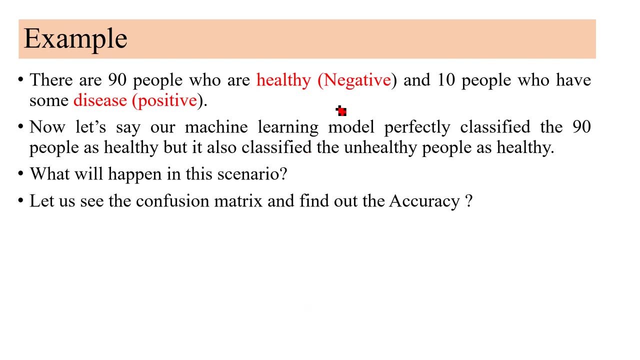 balance, we have to consider the accuracy. so for balanced data set, we have to consider the accuracy. for imbalance data, we have to consider the f1 score. that is the main difference between the accuracy and f1 score. so if you see the one example, there are 90 people. so there are 90 people. 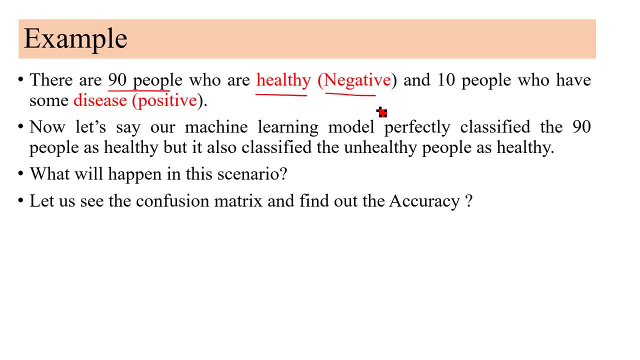 who are healthy means they are no disease, and 10 people who have the disease, totally people are 100. so among the 100 people number of zeros means the number of negative is 90 and the number of ones is positive is 10 people. so let's say, our machine learning model perfectly classified the 90 people. 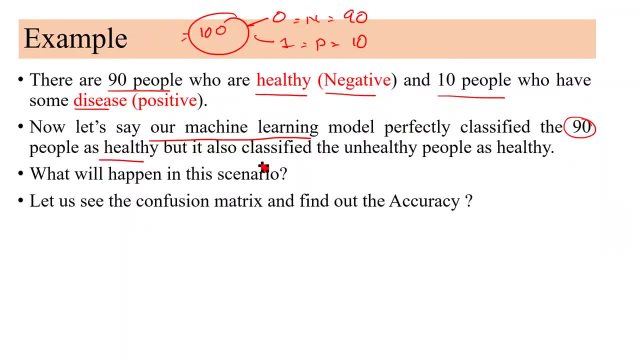 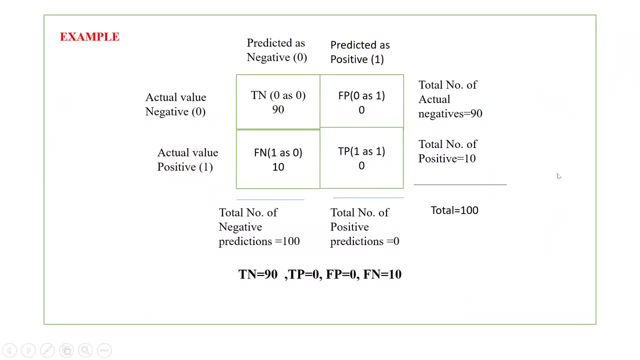 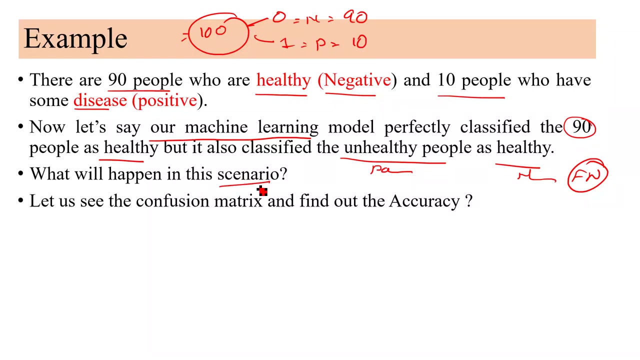 as healthy, but it also classified the unhealthy people as healthy. so unhealthy people means these are the positive people and we consider the negative. so that is nothing but the fn. so this is nothing but the fn. fn. so what will happen in this scenario? so let us see the confusion matrix and find the accuracy. 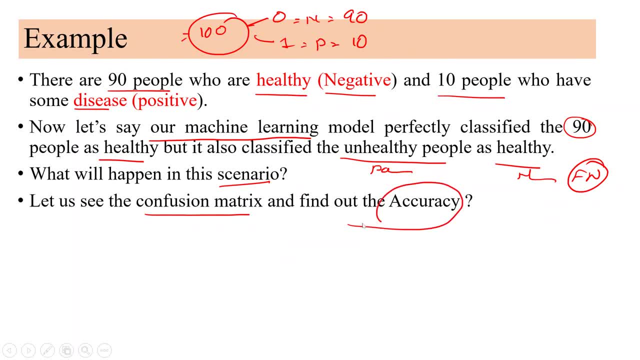 score go. so i will repeat the problem again. so out of 100 people, out of wonder people, 90 people are the negative. negative means no disease. oh, this is means these are the healthy people and 10 people are the positive. positive means you have the disease. so me in this data. 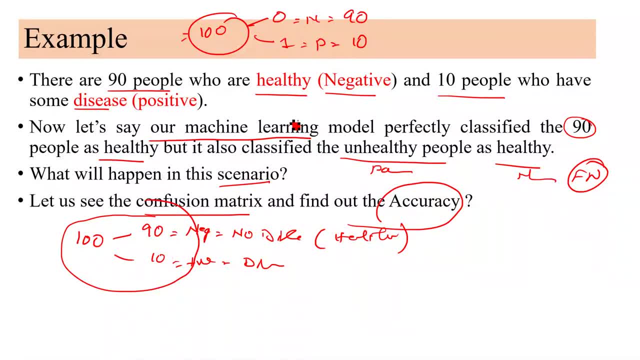 set our machinery model classified the, this 10 people be considered as the healthy people. actually, these are the positive people. we are suffering from the disease. this disease people is the positive people will be considered as the negative people means this is considered the wrongly means that is the false negative. so what will happen in this scenario? so see, 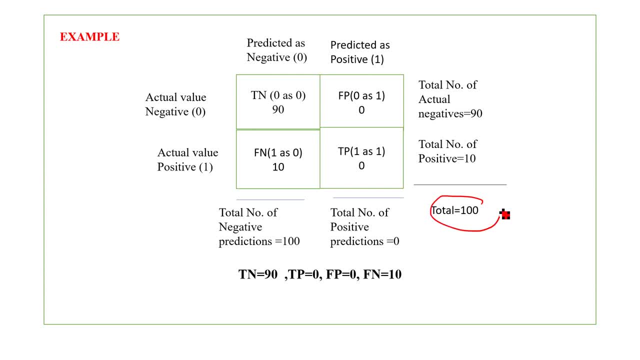 actually total 100 people. among the 100 people, true negatives: 90. so there is no fe, there is no nephew, so total negative people are 90. total negative people are 90 means total number of people, healthy people. healthy people are 90 people and 10 people are the positive people. 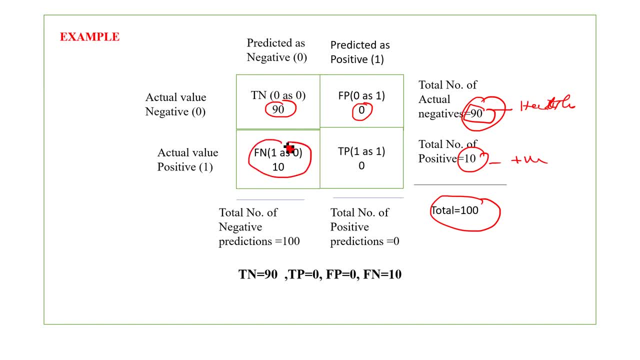 people. positive people means that is the wrongly predicted as the negative. so means the true negative is 90, tp 0. this is tp value 0, there is no tp and there is no fp, and if p 0 and false negative is 10.. so in this case, if you 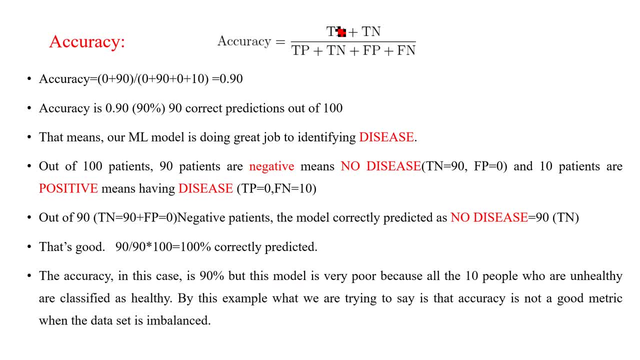 see the accuracy. so accuracy means tp plus tm, means 0 to plus 90 plus this is 90 percentages. accuracy is 90 percentage means after 100 people, 90 people are correct. predictions means that our michelin model is doing great job for identifying the diseases. okay, but out of 100 patients, 90 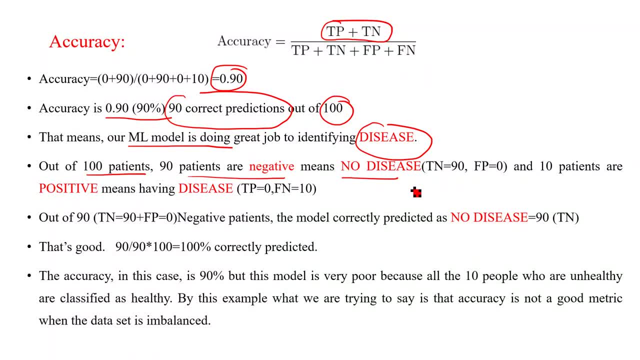 patients is negative means no disease. means 2 negative is 0, fp 0 and 10 patients are the positive means having the disease. so means here tp 0 and false negative 0 is wrongly identified. so means out of 90. after of 90 means 2 negative 0 fp 0 out of 90 negative patients means healthy.